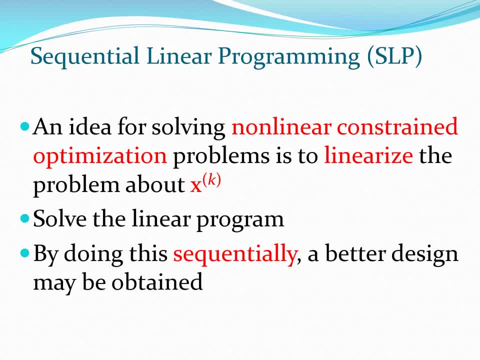 So if we are going to solve a non-linear, constrained optimization problem, why not linearize this problem at a given point x of k and then solve the linear sub problem as a linear program? So we now know that linear programming is a very well developed field and there are a plethora of methods as well as computer programs out there which solve the linear programming. 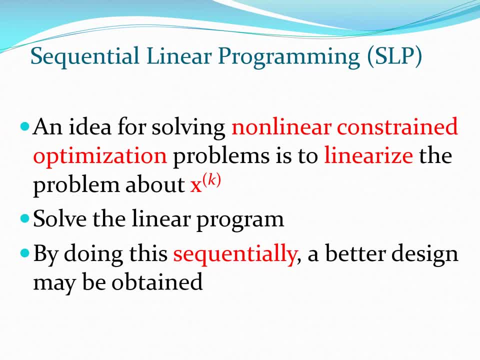 So this looks like a very straightforward and simple way to handle non-linear constrained problems, and therefore we are going to study this in this particular video lecture. Now, of course, you need to use this concept sequentially, because if you are dealing with a non-linear function, if you linearize this function at a point x, k, you are going to get a problem which is a rough. 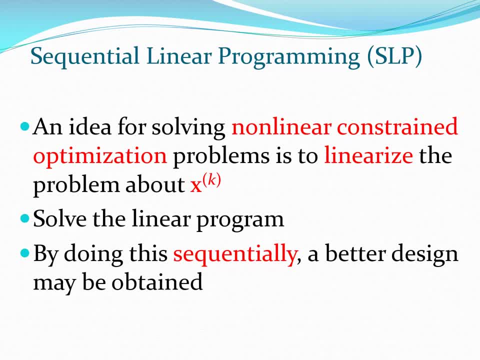 guess of the actual non-linear problem. So if you solve this problem you're going to get a solution, but the solution is not going to be the actual solution of the non-linear constrained optimization problem. But you can use this particular solution as the next point- x, k plus 1- and you can once again linearize around this new point and keep doing this still. 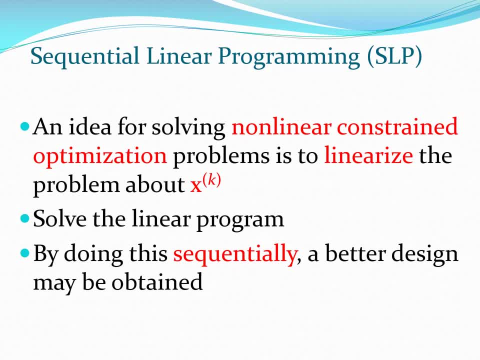 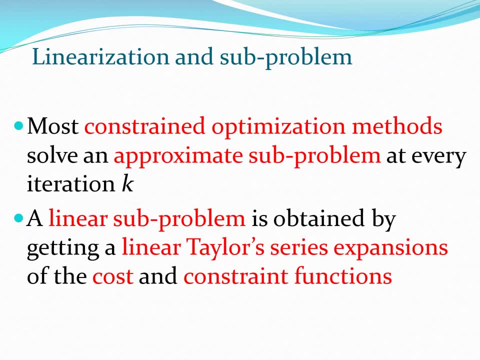 You get a pretty good solution for the nonlinear constrained optimization problem by restricting decision to solve this problem and restricting its solution. to look at it how we would consider heures per second optimization problem. Now, in fact, why sequential linear programming is important? because there are many constraint optimization methods which seek to create a sub problem which is a 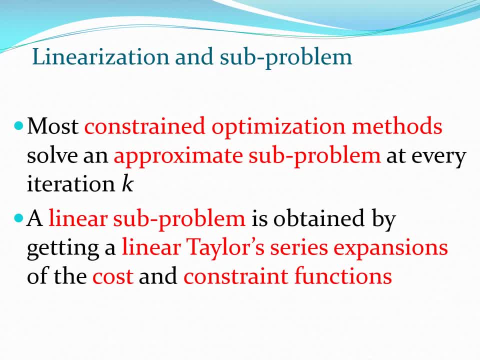 kind of approximation of the actual non-linear programming problem. Now this sub problem could be linear or it could be quadratic. we will later see that a quadratic function or a quadratic problem is a good guess for a real non-linear problem. but as a first stage we can even think: 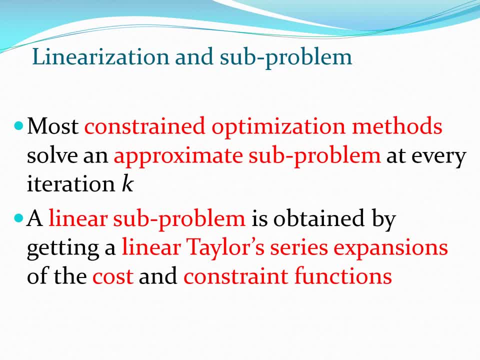 of a linear problem as a good guess for a mildly non-linear problem. So the main task is that you need to create these sub problems at each point k. Now, if we develop a linear sub problem, then we would be using linear Taylor series, expansions of the cost and constraint function. 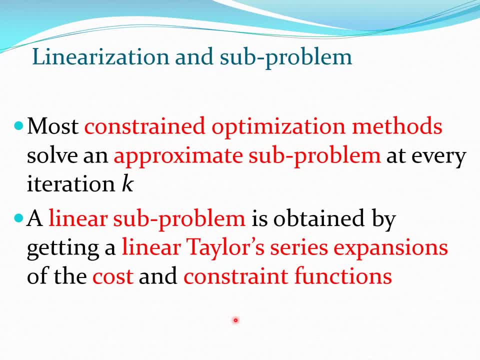 and therefore this kind of linear approximation is going to be valid only very near the point xk, and then we are going to work around that small region and try to find the minimum point at that region and then move beyond from that region. So that's the basic philosophy behind sequential 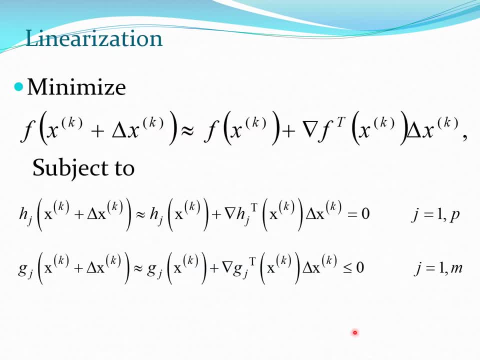 linear programming. So let us do this particular Taylor series approximation. So let's start with the cost function itself. So we take the function f of x and we take a Taylor series and retain only the first term. So you recall that you would have the function value at xk, you would have the gradient of the 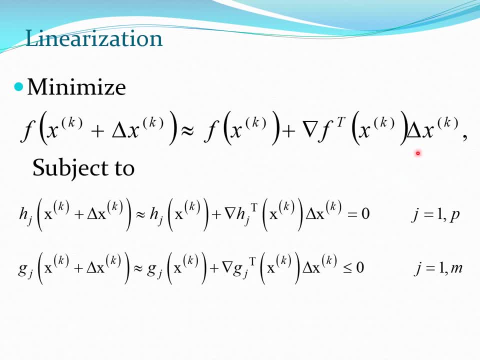 function at xk and you would have the delta xk which is the move in the design space. So essentially, you are at a given point xk and you want to move this delta xk value in the design space to get to the new point. So we form this Taylor series. for the function f, we form one more. 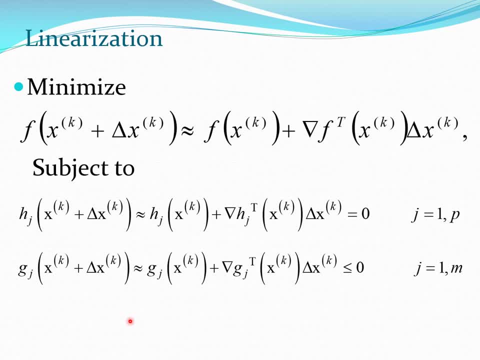 Taylor series for the function h and we form one more Taylor series for the function g. So again, in the case of h and g, you are going to have 1 to p number of equations and you are going to have 1 to m number of expressions here. so again, once you have done, 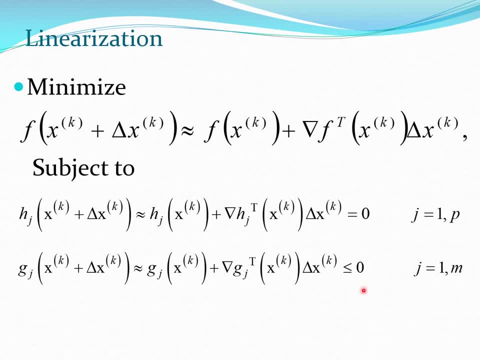 all this, then we would have a linear set of problems, and what we are going to do is we are trying to define, we are going to define some nomenclature so that we can write this whole thing in a simpler form, so we don't have to carry this delta x and so on. so we are going to define. 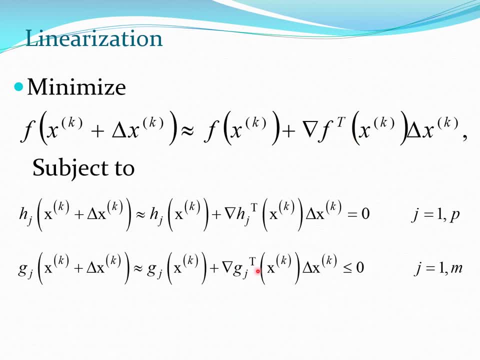 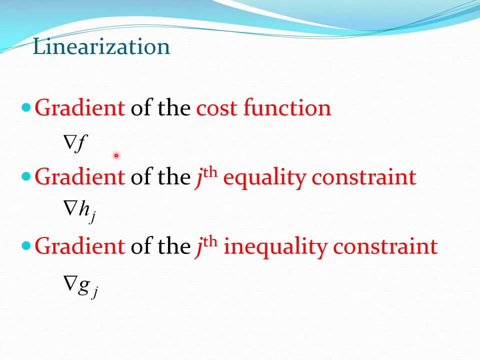 delta x as d, and we are also going to define these gradient values. and we are going to define these particular values at the point x, k, for f, h and g. so we have seen that there are three key gradients here: the gradient of the cost function, the gradient of the h function and 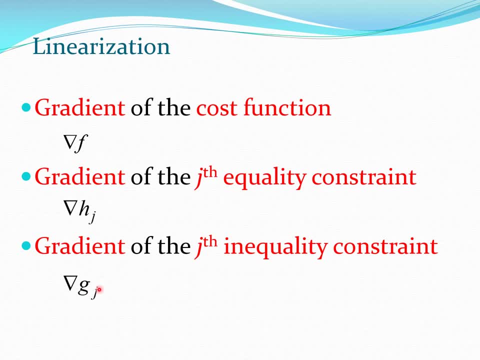 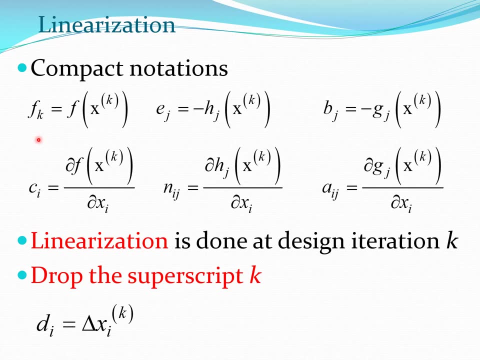 the gradient of the g function which we have obtained from the given problem. so so now we define some of this compact notation. so, for example, we define f, k is f x k, we define e, j is negative, h, j, x k, b j is negative, g, j, x, k and we define the components of the gradient vector. 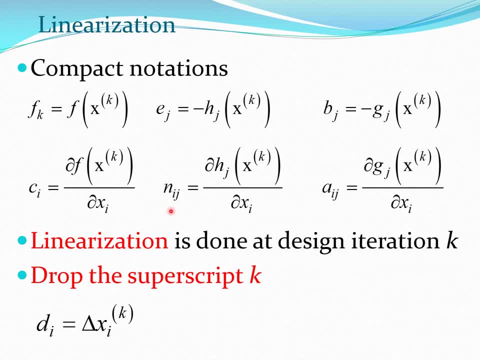 as well as the components of the matrices which contain the gradients of h and g. so this, of course, we are familiar with. so we are going to define some of these gradient values. and this is kind of a great idea because, if you are familiar with from our previous study in terms 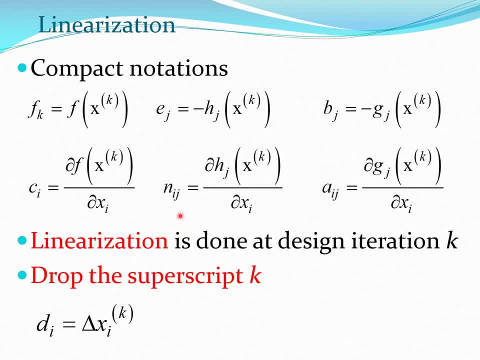 of the vector c, which contains the gradient of the cost function. these are new in terms of gradient of the h functions and the gradient of the g functions. now, here these are actually matrices, because you would have a value n- i- j, which would be dou h- j, by dou x, i, and similarly a i- j would be. 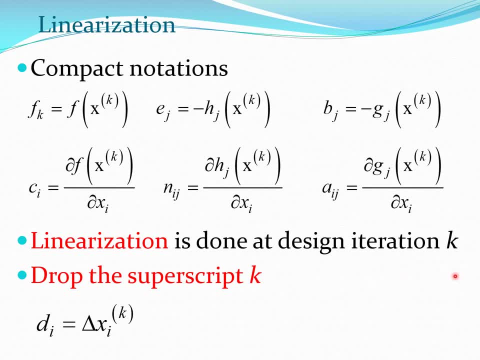 dou g, j by dou x, i, these functions, and so you can haveSteamtimes in the inner twenty structures to the dou xi, and linearization is done at the design point k. again, since we know we are doing all this at sub, at the point k we drop this superscript k, so we are carrying out all these k throughout. 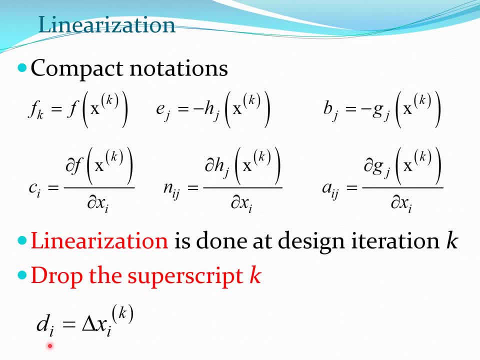 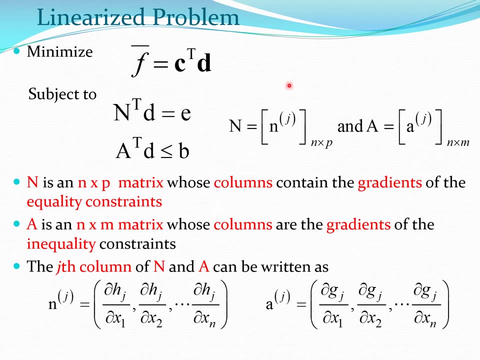 we'll just drop that. so we will simply say that d i is delta x ik. so once we have done all this notation, we can write this linearized problem in a much nicer form. so the problem becomes: minimize this function. f bar is c t d subject to n t d equal e. 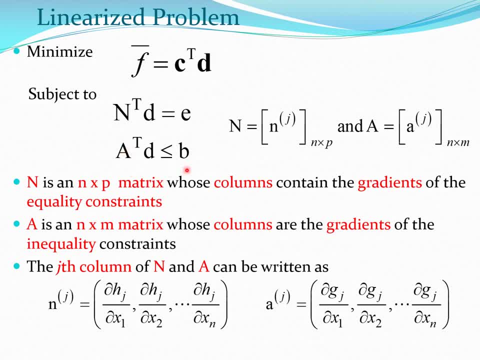 and a, t, d is less than equal to b, where f bar is an approximate objective function. because it is linearized, it is c, t, d, where c would be the gradient vector for the function at the given point and d, of course, would be the search direction we are trying to find. 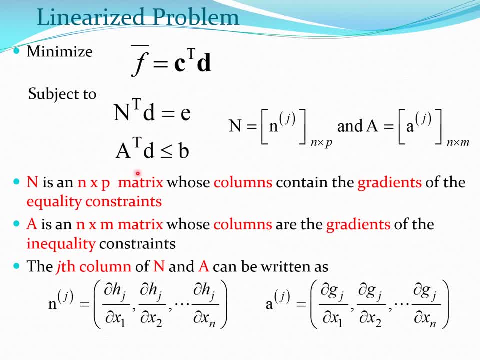 similarly, we would get these two expressions here now: n is an n by p matrix, whose columns contain the gradients of the h constraints. a is an n by m matrix, whose columns are the gradients of the g of x constraint. and so this n, j and a? j are basically derivatives, and so we can calculate them. 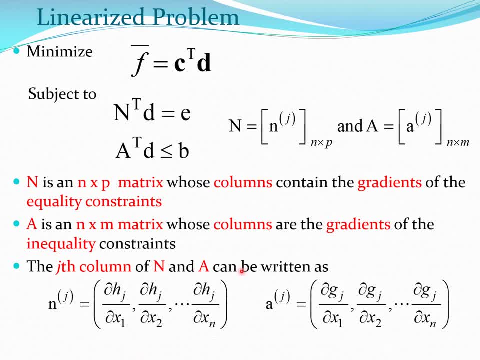 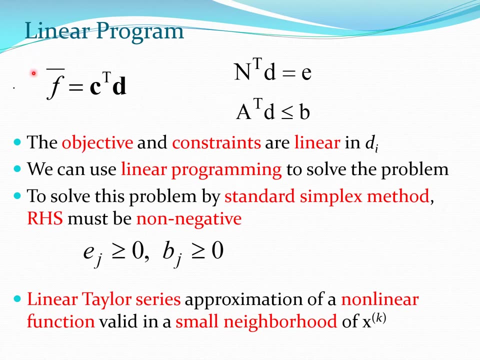 as part of the solution process and if we have taken all this derivative information, we have got this linearized sub problem and now we are going to try to solve this linearized sub problem. so you, so this linearized sub problem is minimize this function. subject to these two constraints. 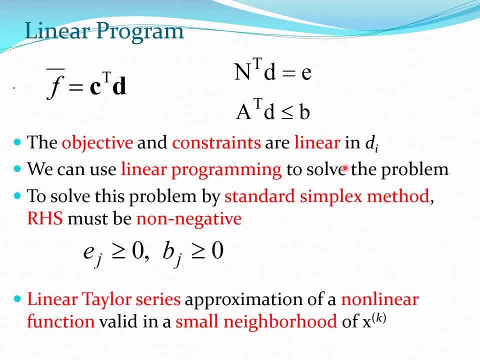 and we clearly see here that because we have taken the linearized taylor series- expansion, the objective function and the constraints are linear in terms of design, variable d- we can use linear programming to solve this problem. now, if these coefficients- here e and b- are greater than 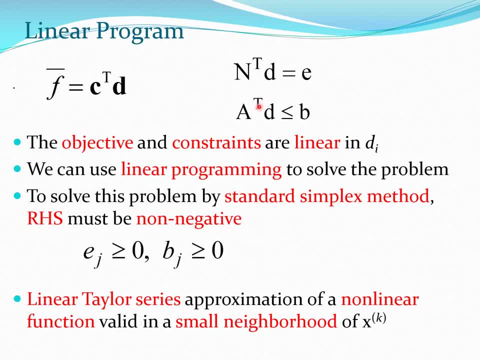 zero, we can use the standard simplex method. of course, if you have greater than type of constraints here, then you can use the two-phase simplex method, define the avs and so on. but anyway, since this is a linear program, you know how to solve this problem, either by yourself or by taking records to the numerous software packages which 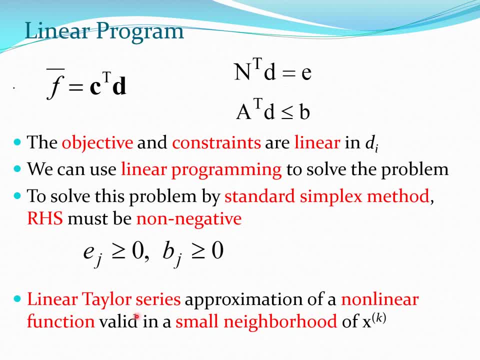 are out there in linear programming. now remember that this linear taylor series of a non-linear function is only going to be valid in a small neighborhood of xk. and this is where the problems of sequential linear programming start coming in, because this particular linear sub problem which we have developed may work only in the small 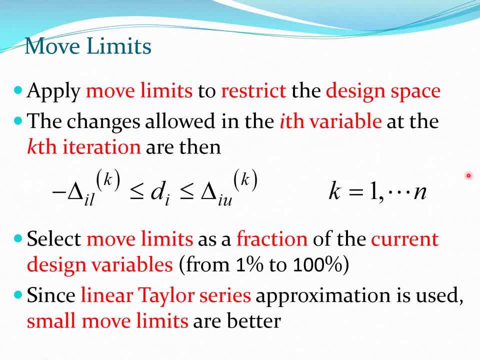 neighborhood of the point xk. that is why the concept of move limits becomes very important in sequential linear programming and essentially we put move limits on this design variable di, which is basically the level of movement. we have permitted this problem in the design space. so these move limits, 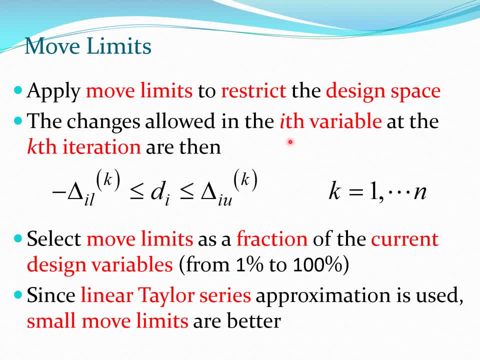 are used to restrict the design space. so, for example, if we have di, we say this should be greater than some value here and it should be less than some value here. so that's a typical move limit which is put on this kind of design variable. now this is put for all. the k is 1 to n variables here. 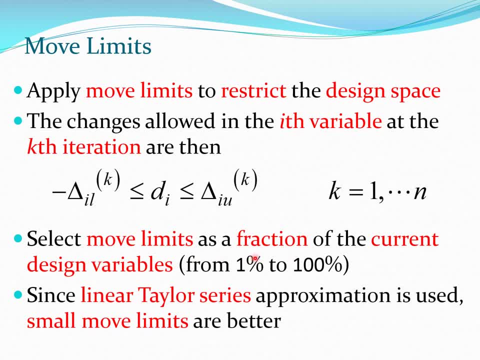 now the move limits typically can be selected as a fraction of the current design point. so you may move by 1 to 100 depending on the level of confidence you have in your linear taylor series expansion. now typically you can understand from mathematics and calculus that because you have 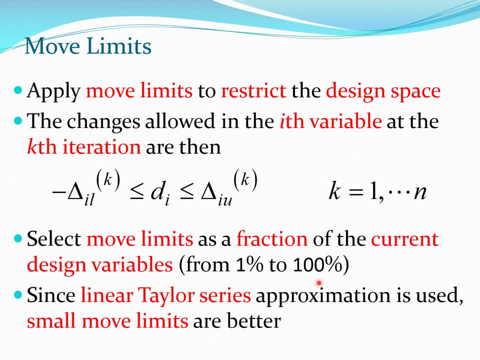 used a linear expansion, and if your function is not too non-linear, then you need to take small move limits. if your function is not too non-linear, then you need to take small move limits. if your function is very non-linear, this method is probably going to be problematic, so let us presume that 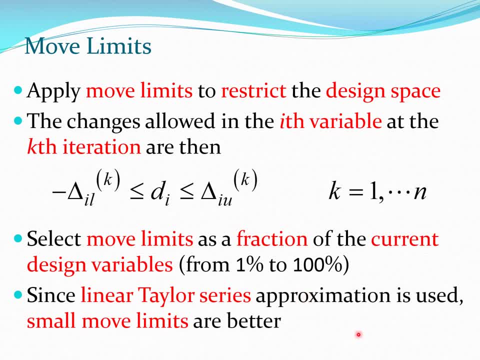 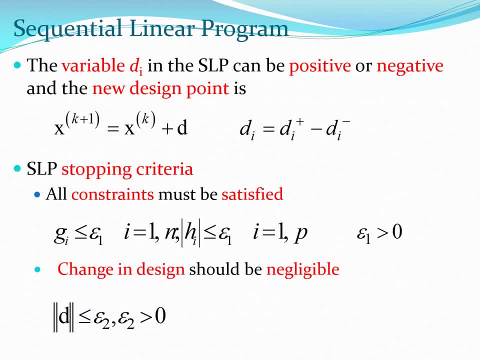 your function is mildly non-linear and then taking small move limits may help you to actually converge to a solution using this particular method. so we also recall that the next point is going to be: xk plus 1 is xk plus d. remember that d is delta xk, so therefore it is the movement you make in the 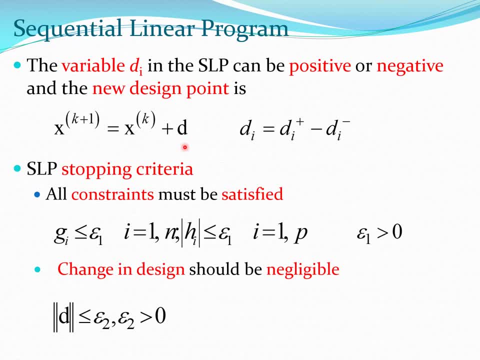 direction. so essentially, you are using the sequential linear program to move in the design space. and also this variable, di, can be positive or negative. so, again based on the theory of linear programming, we have to split it into two different variables, both of which are positive, and then we 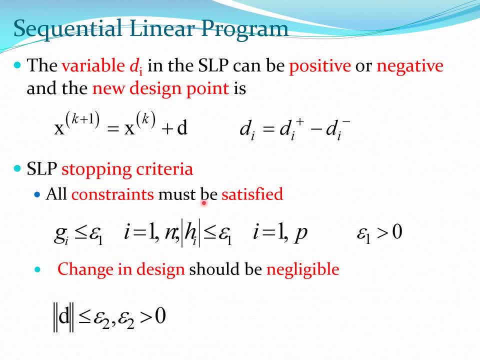 can solve this problem now. some of the stopping criteria which can be used for the sequential linear programming are as follows. number one is that all your constraints must be equal to the number of constraints and number of constraints- sorry state. it needs much more Athenian into D. 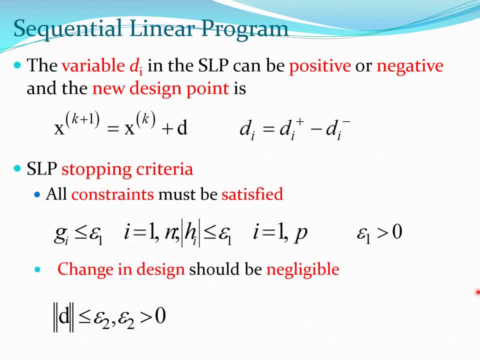 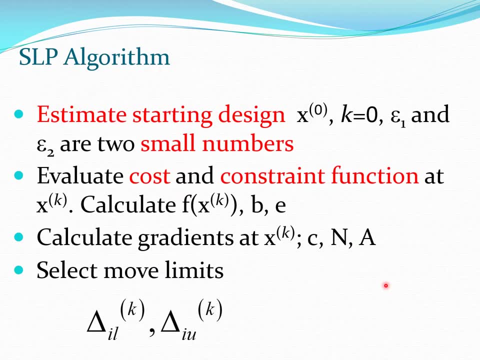 to below that particular number. this number could be 10 to the power minus 4 or 10 to the power minus 8, for example. so let us now write down this method in terms of a pseudo code which you can use to program. so we start with the starting design. so of course, that is required in all. 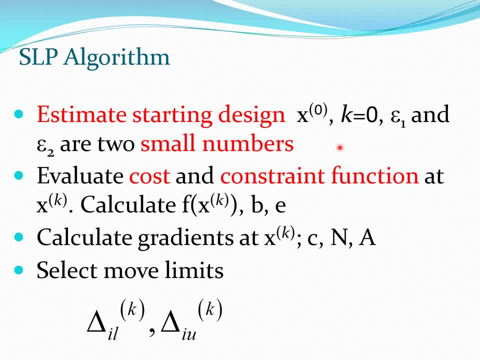 these type of methods. so the starting design is x: 0, this is k: 0. select two small numbers. find the cost and constraint functions at point xk. calculate the function value at this point and also the b and e values. now calculate the gradients at xk. so for the cost function you get. 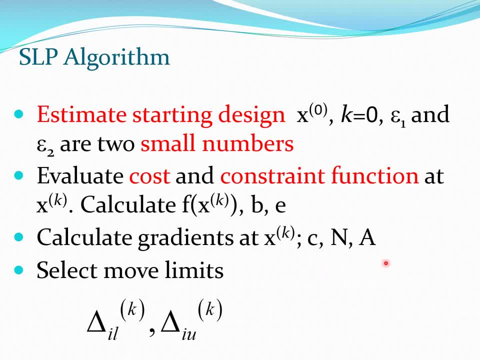 c and for the constraints h and g you are going to get n and a matrices. now you select the move limits on this particular value to move in the design space. so this is a lower limit, this is a higher limit and you can select these. now you define the lp sub problem. you solve for d of k. 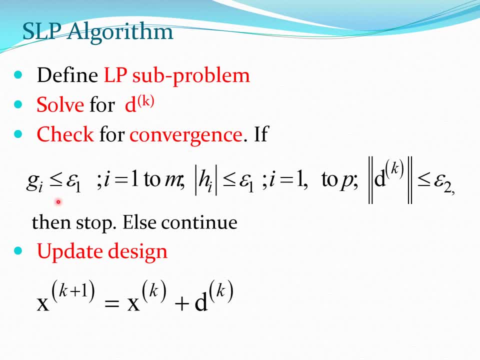 check for convergence. so the check for convergence is simply that your constraints must be satisfied and also your design has more or less converged, so you are no longer moving in the design space. if this has happened, you can stop, else you continue the process, you go to a new design. 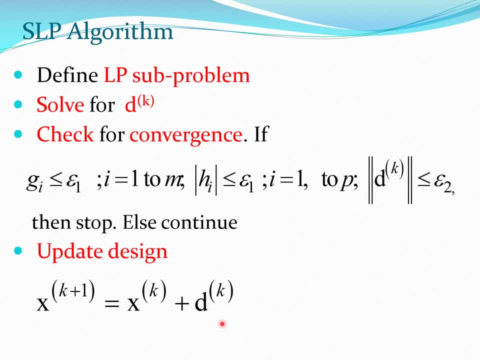 and so on. now the trick in sequential linear programming is to progressively relax the move limits as you go through the process. so when you start with the low value of k, your move limits are pretty tight, and then, as you are becoming more and more confident of the progress of your method, you 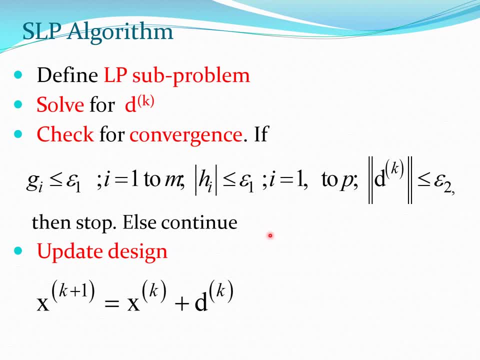 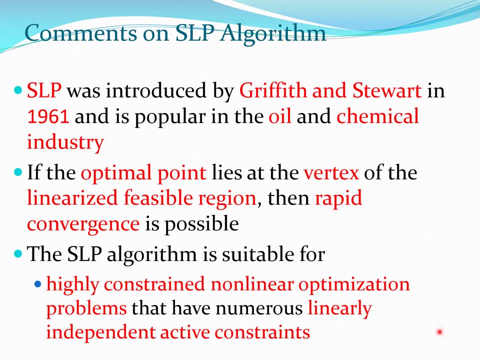 start relaxing the move limits, and if you are able to do this well, then you will converge with this particular method. so sequential linear programming was actually developed by griffith and stewart in 1961. it's popular in the oil and the chemical fields. if the optimal point lies at the vertex of the 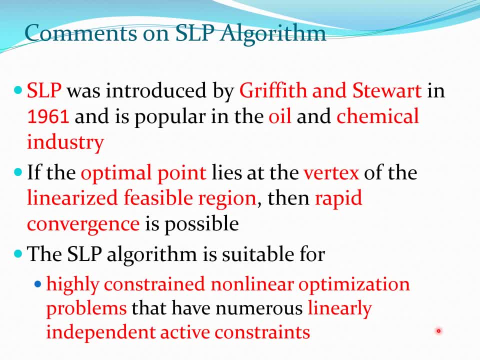 linearized feasible region, then rapid convergence is possible and this you can understand from our previous study of linear programming. now this method is suitable for highly constrained non-linear optimization problems where you have numerous linearly independent active constraints, and if you have a particular problem which defines some of these things, or 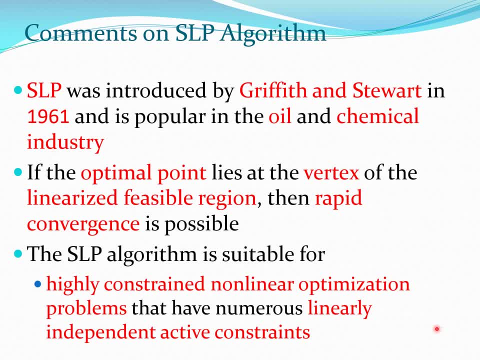 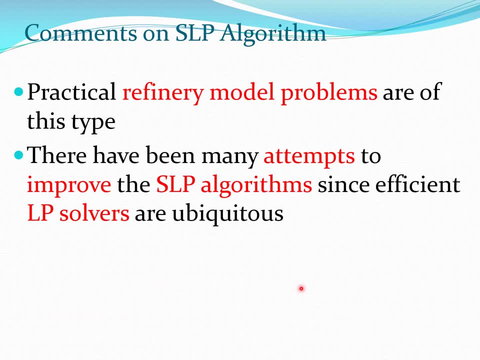 which satisfies some of these conditions, then you may do well with this method. so one of the important practical problems of this type are found in refinery model problems and that's where this method is quite frequent used. now you can imagine that many people or researchers have tried to improve the method from. 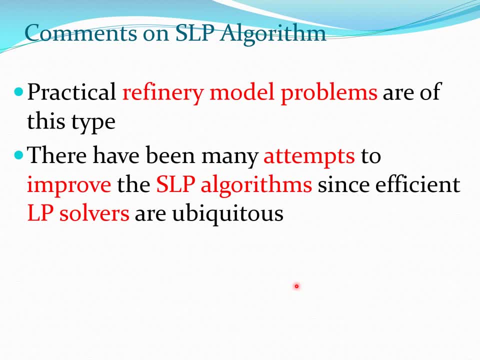 what we have given here. so what we have given here is a very basic outline of this method. now, one of the reasons to improve this method is that the linear programming solvers are very popular and widespread and therefore you can use these linear programming solvers in. 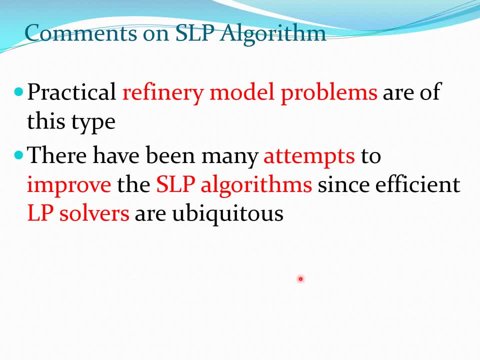 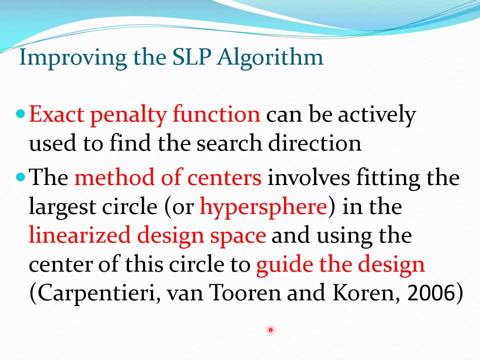 this particular method, so you would just have to do this linearization, you can just do this linearization and you can do this linearization. now some people have suggested that you can use a penalty function to actively guide the search direction, so we have discussed some such penalty functions before. there is also this method of 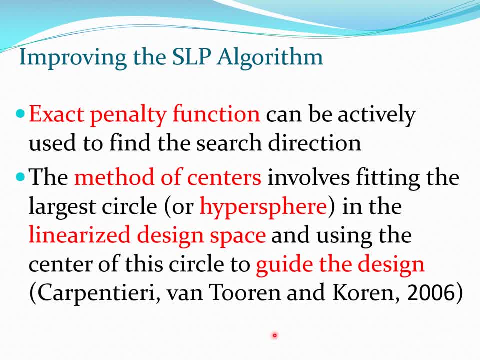 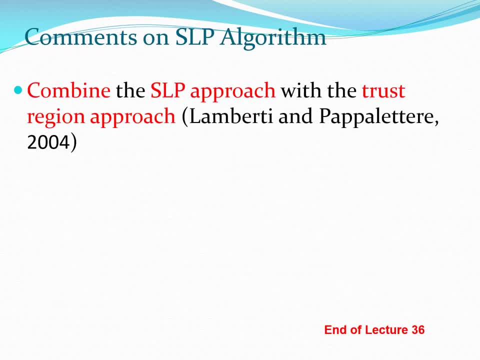 centers, which basically requires you to fit the largest circle in this linearized design space and use the center of this circle to guide the design. this was proposed by some researchers. You also could combine, combine the sequential linear programming approach with the trust region method, and trust region method basically tries to define a region around your point XK which you can trust in the sense that where the approximation which you have developed is valid. 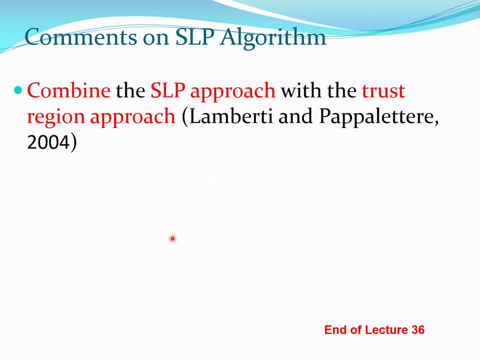 And so if you are able to trust in the nearby region of XK that your linear approximation is valid, then you can be in this particular region and move step by step in a sequential manner towards the actual solution. So that would make a lot of sense is to combine this kind of method with the trust region method, and that has been proposed by some researchers. I think we are going to discuss trust region methods in a later lecture.